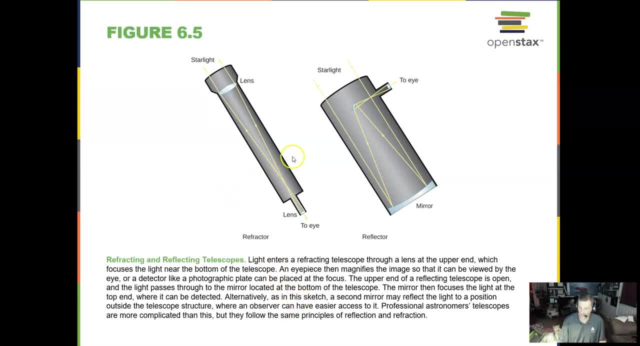 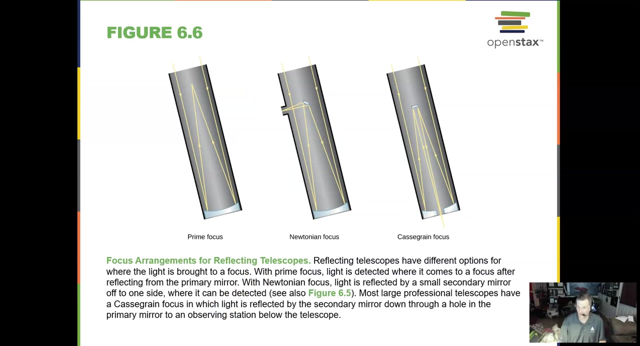 basically, refracting telescopes spin light through a lens, a glass lens, Whereas a reflecting telescope reflects light off of a mirror through another mirror. Then it goes to an eyepiece, which is a lens. You can have different areas of focus in a reflecting telescope. 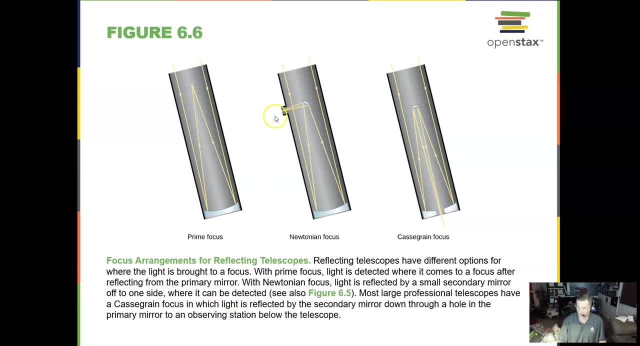 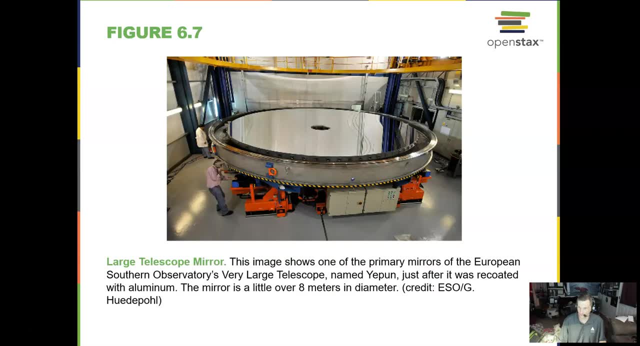 You can have it coming out of the aperture, the eyepiece or a focus within the mirror itself. Here is a very large telescope mirror. This is going to go on the European Southern Observatory's Very Large Telescope. We like to name our instruments and telescopes interesting names. 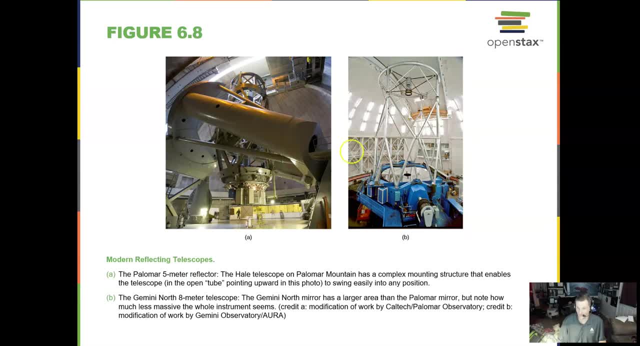 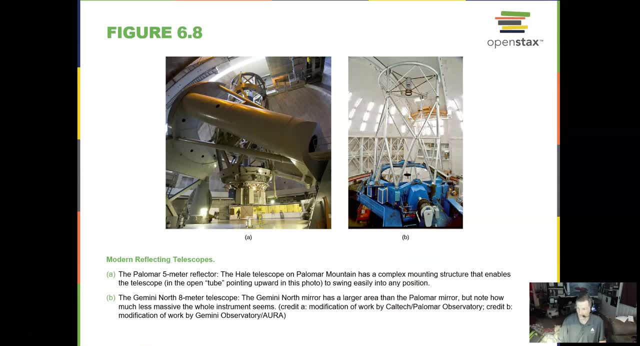 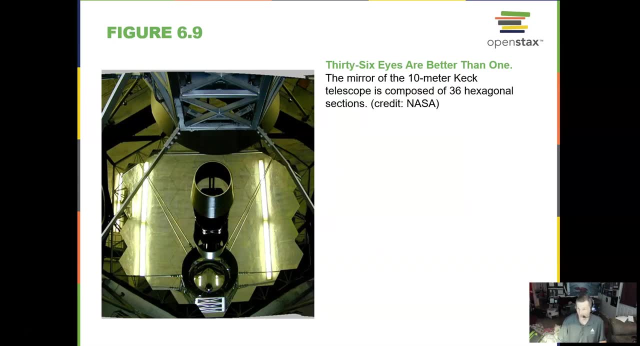 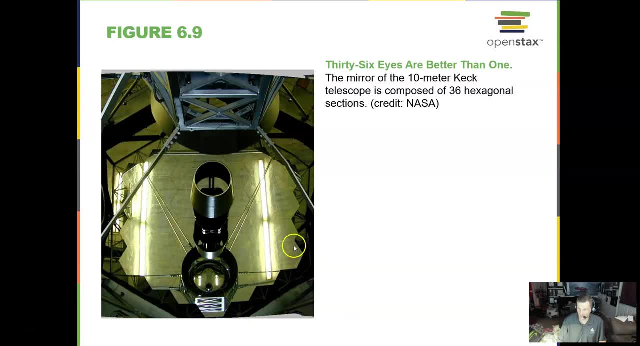 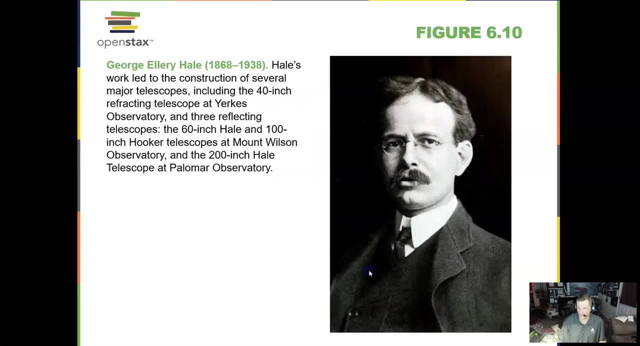 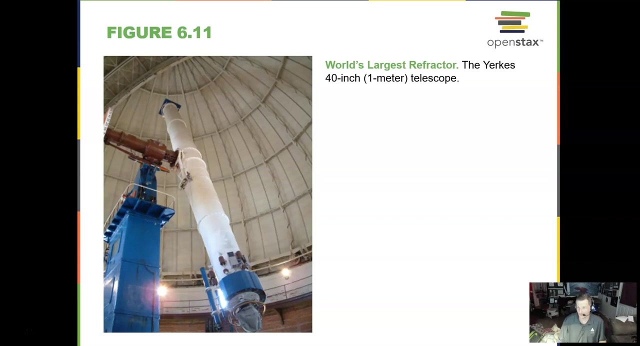 In order to build a compact but very large telescope, we can use segmented mirrors. The segments here are all glued together to make one large mirror. This is for Keck Telescope in Hawaii. This is for Keck Telescope in Hawaii, But George Hale led to work of the construction of several major telescopes: the largest refractor, 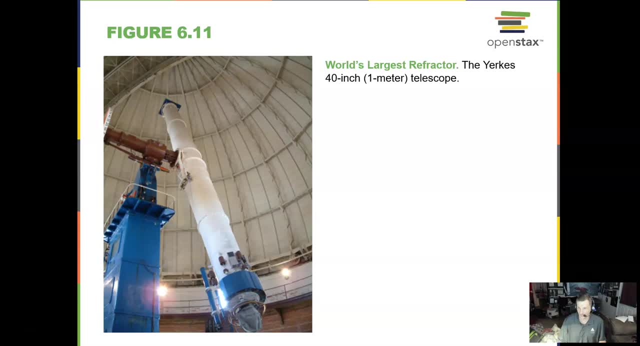 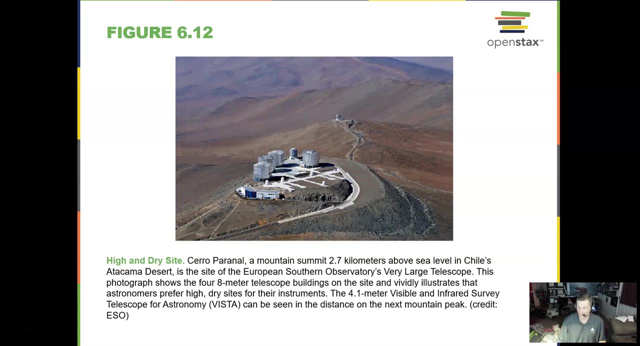 bending telescope in the world is a 40-inch, and this is in Chicago. Most observatories are put as far high up on a mountain as they can go. Here we have a high and dry site at Chile's Atacama Desert, part of the European Southern. 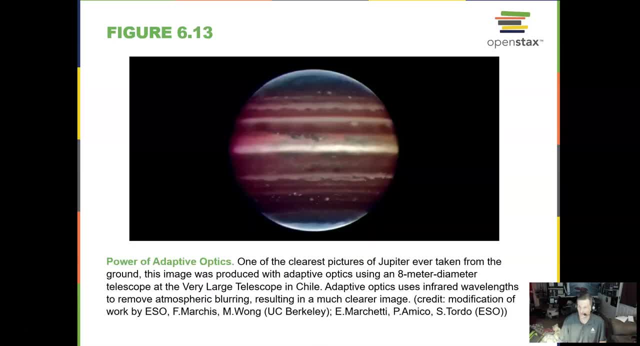 Observatory. Now we can put pistons on the back of these telescope mirrors and these pistons can move the mirror ever so slightly to correct it for the atmosphere, and that's called adaptive or active optics. Here is a picture of Jupiter with those active optics working and you get a great image. 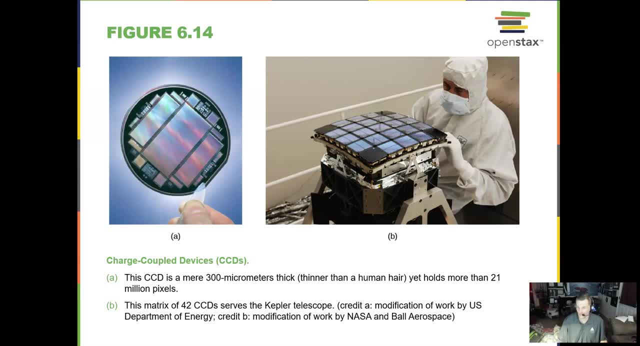 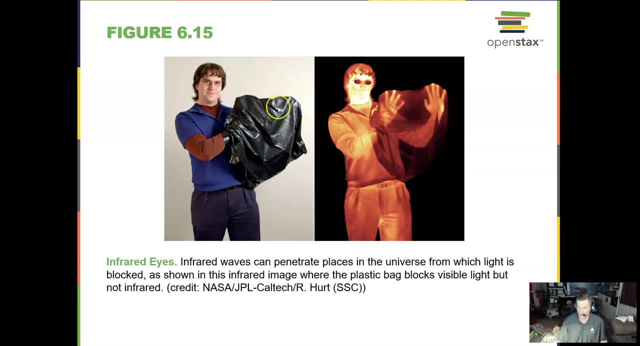 The backbone of these cameras are these CCDs. they're called charge coupled devices, and that's basically a silicon wafer that is sensitive to light- Infrared Infrared. We can see these hands in the bag very clearly in the infrared. 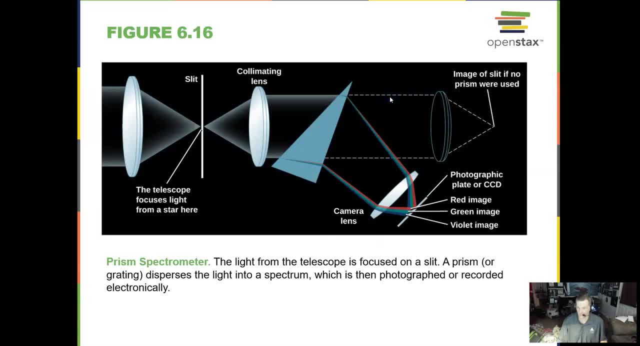 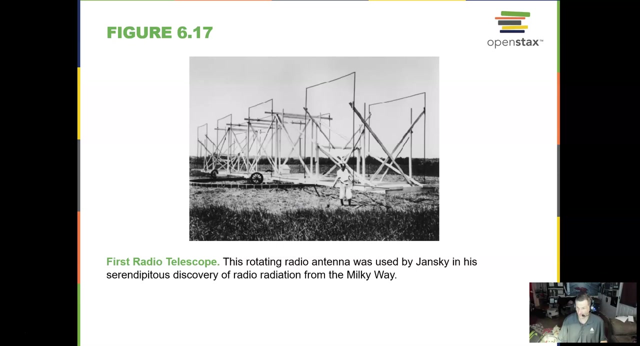 Infrared gives off heat radiation In a prism spectrometer. this is an instrument that will split up the light from white light into its colorful rainbow pattern. Here's the first radio telescope. very basic, This telescope was used by Jansky in his discovery of radio radiation from the Milky Way. 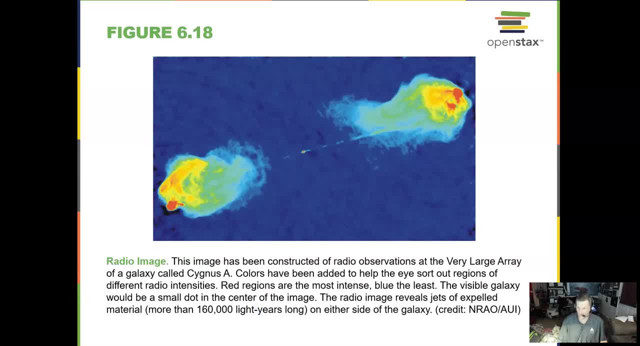 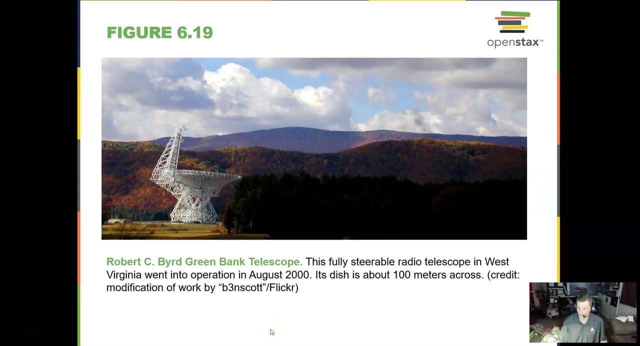 And this is what a radio image looks like. There is a galaxy right here in the middle that doesn't give off very much radio information. They're coming off two lobes Far out, Far out into space. We see jets coming from this image. 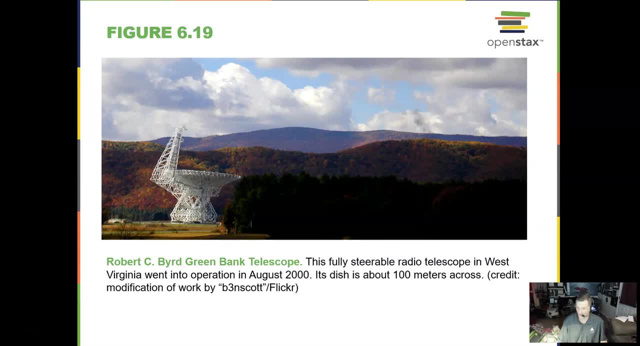 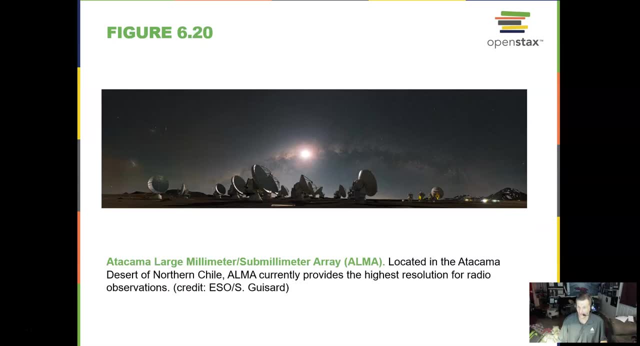 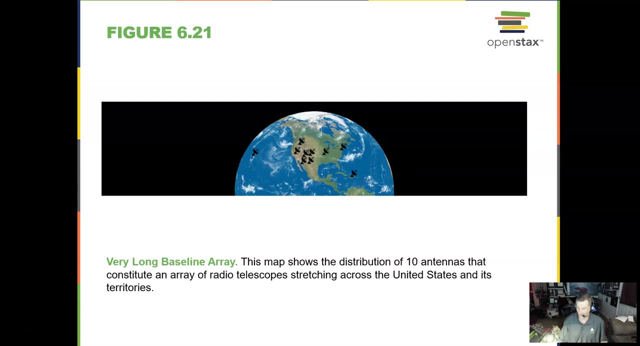 The Green Bank Telescope in West Virginia is pretty large, 100 meters across The Large Millimeter Array in Chile, The Atacama Desert again in Northern Chile. Or you can put radio telescopes throughout the Earth and link them all together so that